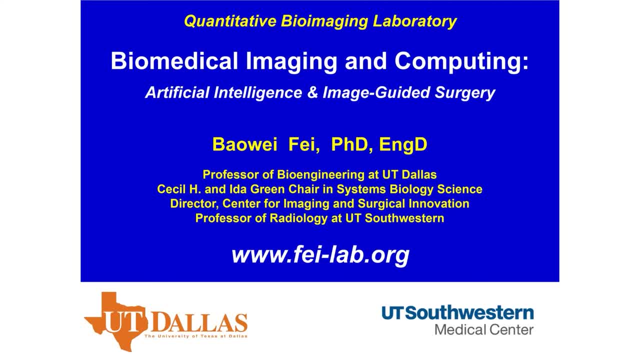 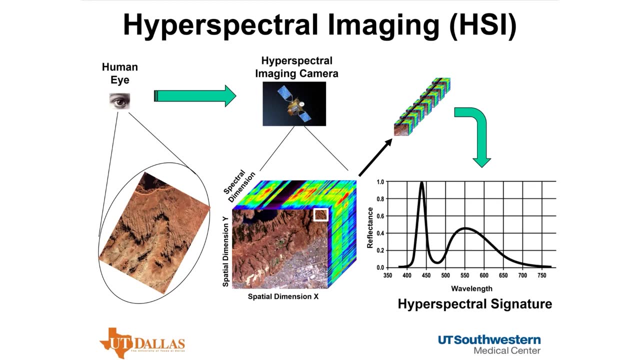 Our research project involves imaging, data science, artificial intelligence and image-guided surgery. I will briefly cover a couple of projects. One of my research areas is called hyperspectral imaging. This is a technology that was originally developed by the University of Texas at Dallas. 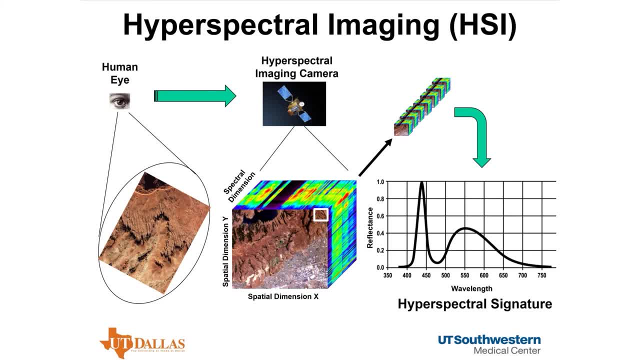 It is a technology that was originally developed by the University of Texas at Dallas. It is a technology that was originally developed by the University of Texas at Dallas. It is a technology that was originally developed by NASA for Earth observation. We are using this technology for biological and medical application. 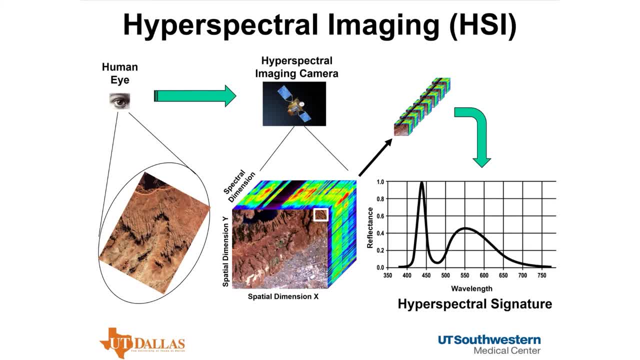 This is not trivial, because we are looking at the cellular and molecular level, and it requires very high spatial resolution and high sensitivity. As you can see, each pixel has a spectral signature that can be used to detect disease. This is a very important feature of hyperspectral imaging. 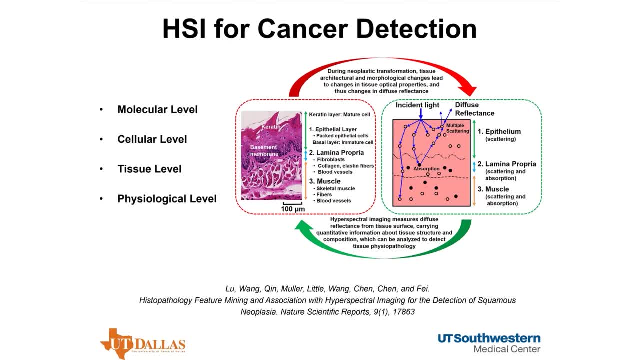 So what is the premise of using hyperspectral imaging for cancer detection, for example? During the neoplastic transformation, tissue architecture and morphological change lead to the change in tissue optical properties and lead to the change in diffuse reflectance. So hyperspectral imaging measures the diffuse reflectance from tissue surface. 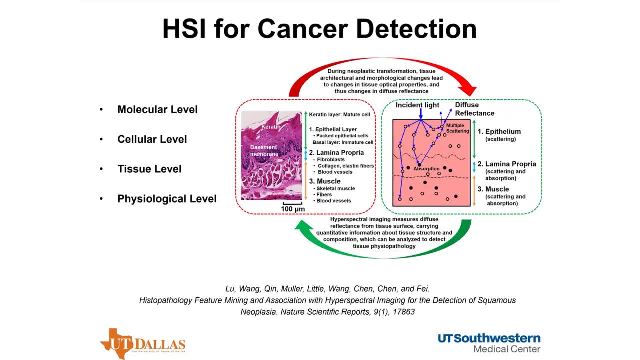 If we look at cancer tissue and the benign tissue, we can see a difference at the molecular level, cellular level, tissue level and also physiological level. These differences can be quite complex. The change in tissue structure and composition can be analyzed to detect tissue pathology. 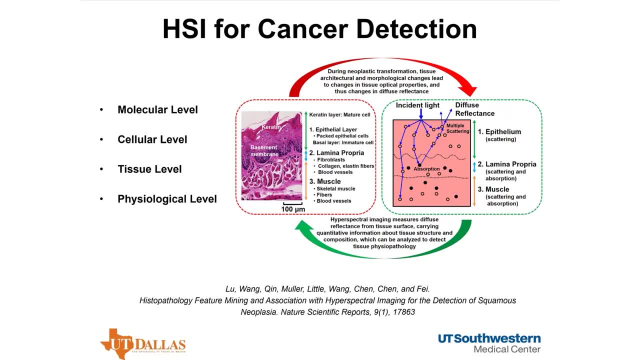 If we look at cancer tissue and the benign tissue, we can see a difference at the molecular level, cellular level and also physiological level. The change in the reflectance hyperspectral imaging can be due to all these changes. This brings some challenges and also brings some great opportunities. 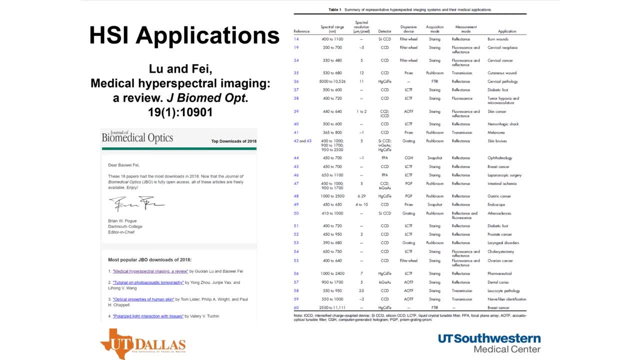 In this review paper, we summarize different applications and different hyperspectral imaging technologies. This is one of the top-downloaded papers from Journal of Biomedical Objects, with more than 1,000 citations. This is one of the top-downloaded papers from Journal of Biomedical Objects, with more than 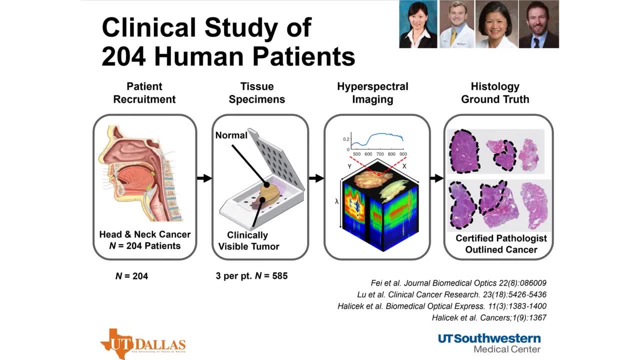 1,000 citations. This is one of the top-downloaded papers from Journal of Biomedical Objects with more than 1,000 citations. In this review paper we summarize different applications and some great opportunities From this resources range. we Tech-Curvesz successful to 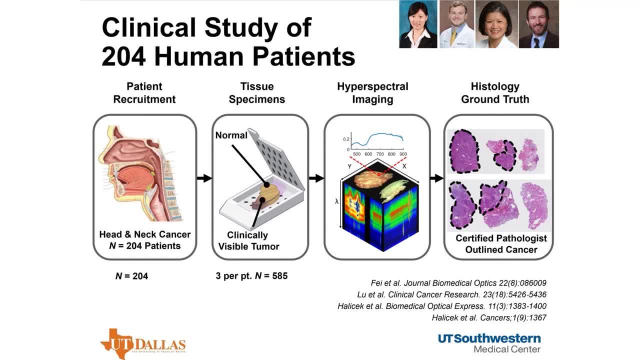 achieve this different licensed behaviour to the tray so that and a pathologist, Dr James Little, on this study. So we recruit a patient who undergo head and neck surgery and for each patient we connected three types of tissue during surgery. It includes cancer tissue, normal tissue and a mix of tumor and cancer tissue. 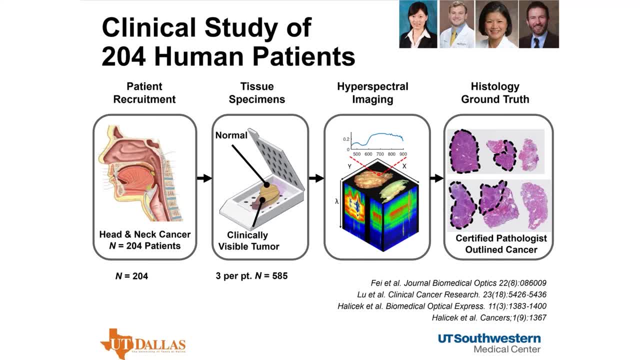 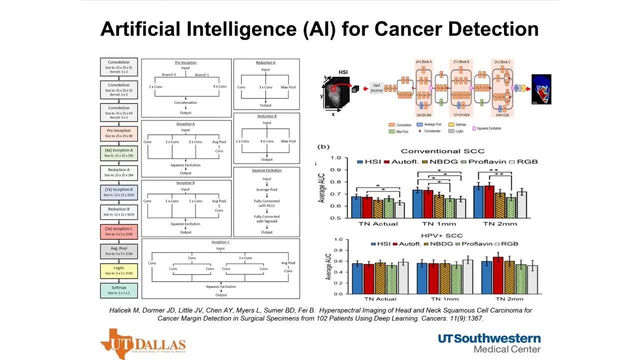 We developed a standard protocol for imaging acquisition of this tissue. We have worked with a pathologist to establish histologic ground truth for each tissue. So we developed artificial intelligence technology for cancer detection. So in this study we use Inception4 convolutional neural network, as shown on the left side. 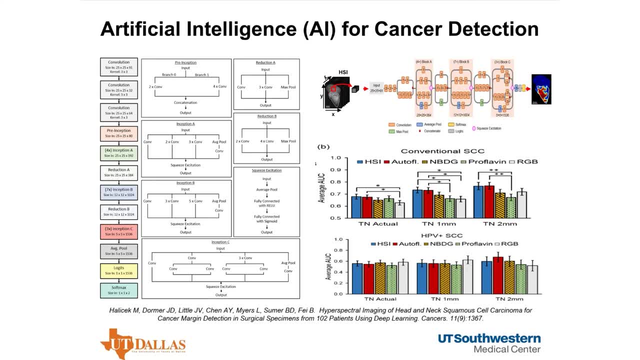 So the CNN architectures are customized. for the hyperspectral imaging cube, We use the TensorFlow, Python and Inverse, We use the NVIDIA GPU and the result shows that the AI algorithms and hyperspectral imaging are able to detect the tumor margin with the accuracies of 90%, and for conventional 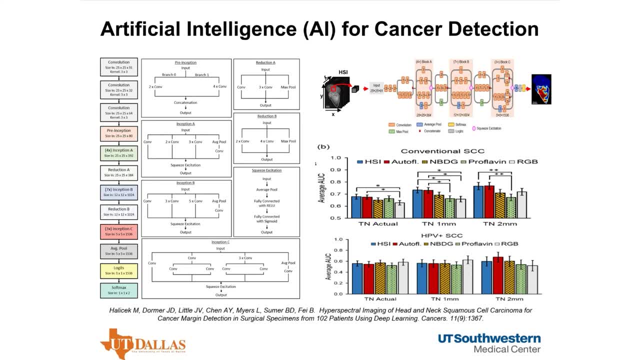 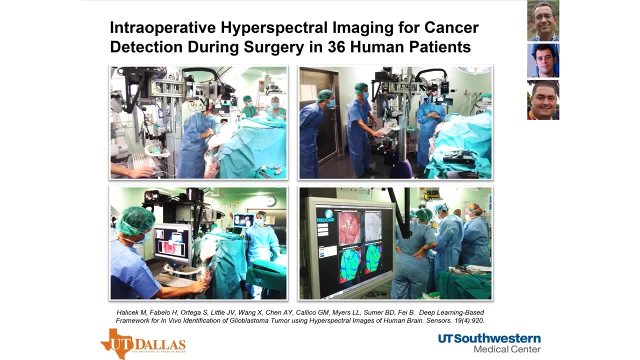 squamous cell carcinoma and 97% for HPV-positive squamous cell carcinoma. That's a very exciting result. So our goal is to use real-time hyperspectral imaging for cancer detection during surgery. We are collaborating with Dr Gustav Karnakos' group, where a demonstrator system has been. 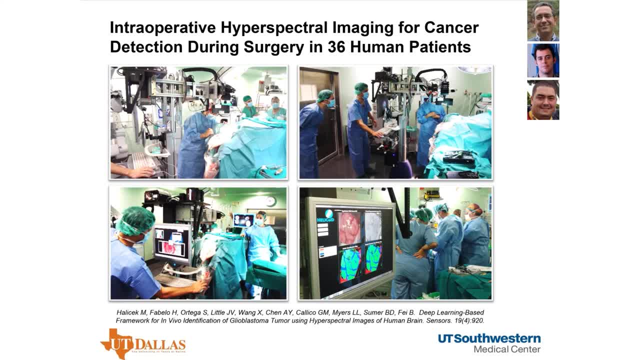 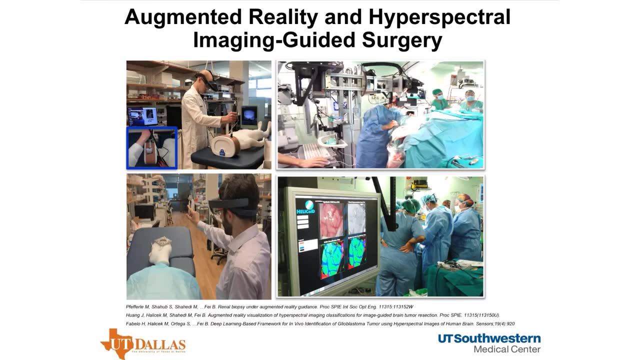 used for brain tumor surgery in 36 patients. We developed a deep learning-based framework for in-vehicle detection of glomerular tumors using hyperspectral imaging of human brains, So we are further developing augmented reality systems for image-guided imaging. Thank you, 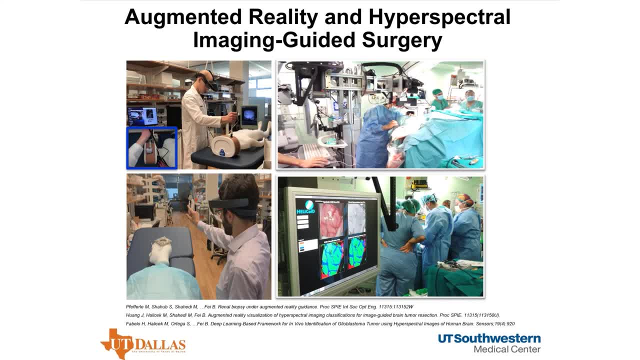 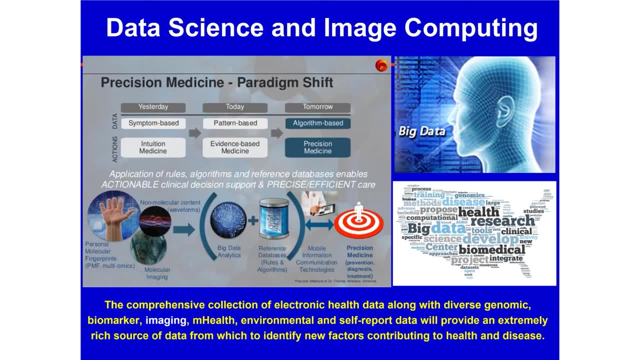 The image on the left side shows the testing of our augmented reality systems, and this is an ongoing research project. Another area in my research lab is data science and image computing. The collection of electronic data, along with biomarkers and imaging, will provide a rich 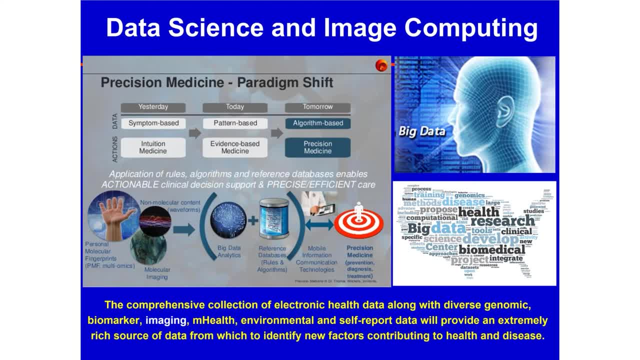 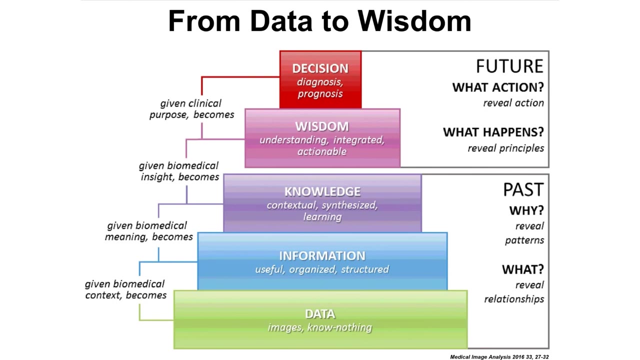 source of data for identifying new factors contributing to hair growth, Contributing to health and disease. So those rich data, plus reference database, plus AI algorithms, will aid clinicians to make early detection, precise diagnosis and a more effective treatment for each individual. So data itself know nothing. however, given biomedical context, it becomes information. 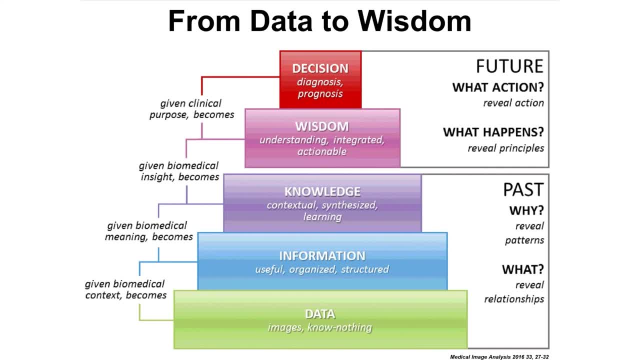 So we can know. Data science should not only be used to identify hair growth, as doctors are doing now. it can also be used to identify the complex relationship of hair growth. Data science is in line with the age of human beings. The data scientist, as soon as he or she sees a result, will know it. 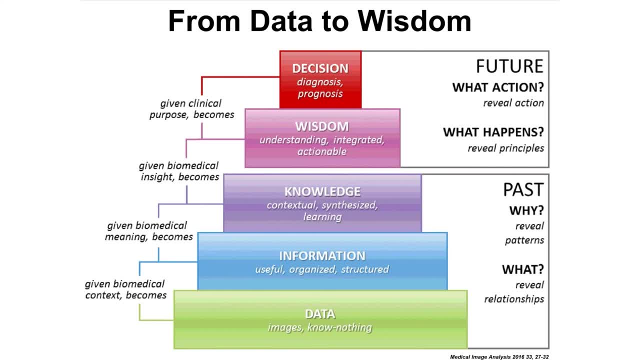 Because of this, we have the ability to compare the difference in hair growth and the hair growth compared to the size of the hair on the side, For example. in this case, the process reaction of the hair growth of a kidney has been more accurate. 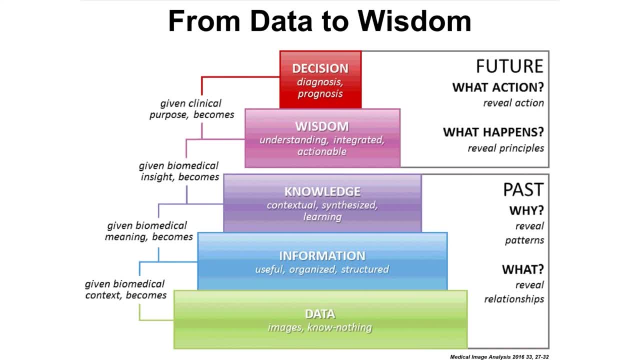 We can compare our experience with the pattern of hair growth. We can also measure the trends in the hair growth. We can see the different amounts of hair growth. We can also measure the distance between hair growth in the vitamin B and vitamin E. help us make clinical decision. you can better treat patient. we even do some. 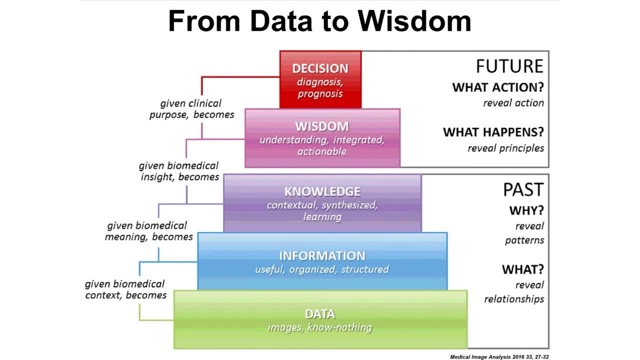 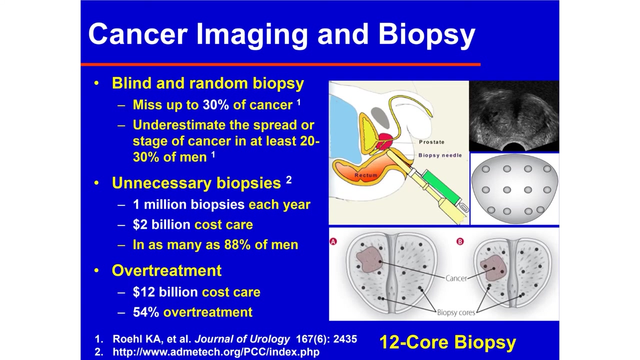 prevention. this is a new paradigm from data to information, to knowledge, to wisdom and to clinical decision-making. in next slides I will give an example on how we use imaging and data for improved a patient care. so one area is the cancer imaging, early detection diagnosis. here we focus on one type of cancer: prostate. 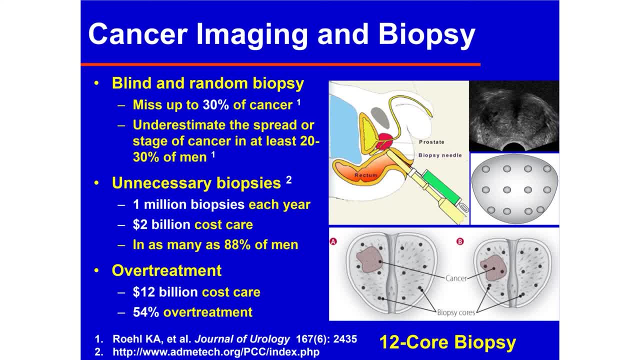 cancer is one of the leading cause of cancer mortalities. the definite diagnosis for prostate cancer is biopsy. there are more than 1 million biopsies each year each year, and the most common cause of cancer mortality is cancer cell cancer biopsy. there are more than 1 million biopsy each year each year, and the most 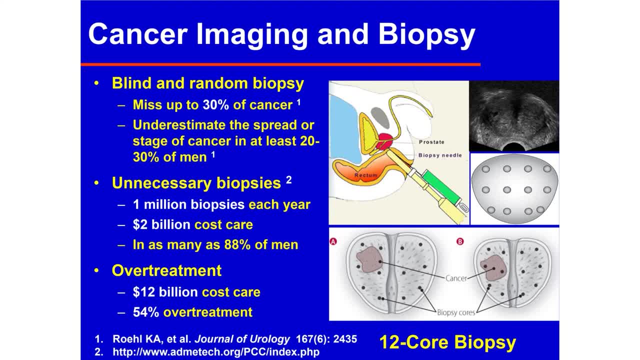 common cause of cancer mortality is cancer- cell cell cancer in the USA in the USA. in the USA transurector ultrasound is used to guide. transurector ultrasound is used to guide. transurector ultrasound is used to guide the biopsy. it is called truss guided. 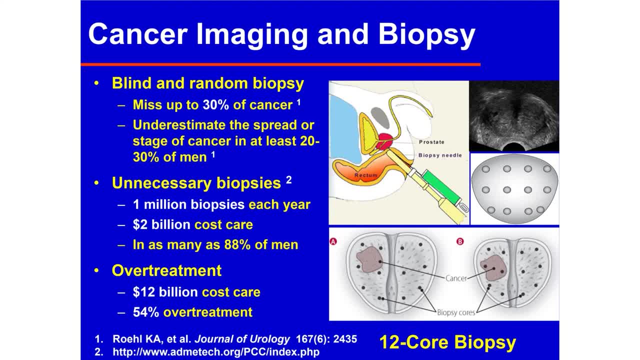 the biopsy. it is called truss guided the biopsy. it is called truss guided biopsy. unfortunately, this is standard biopsy. unfortunately, this is standard biopsy. unfortunately, this is standard truss guided biopsy can miss up to 30%. truss guided biopsy can miss up to 30%. 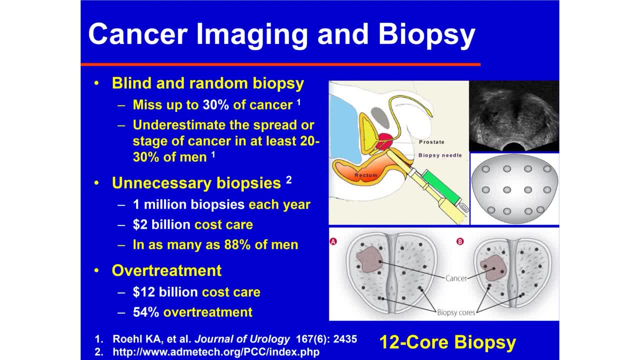 truss guided biopsy can miss up to 30% of prostate cancer recorded blinded of prostate cancer recorded blinded of prostate cancer recorded blinded biopsy. so in this project we develop a biopsy. so in this project we develop a biopsy. so in this project we develop a new imaging method and try to improve. 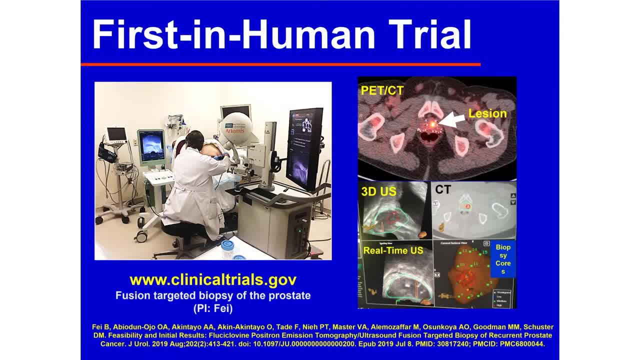 new imaging method and try to improve new imaging method and try to improve my lab combined multiple imaging. my lab combined multiple imaging. my lab combined multiple imaging modality together to guide the prostate modality together, to guide the prostate modality together to guide the prostate biopsy in order to improve detection. 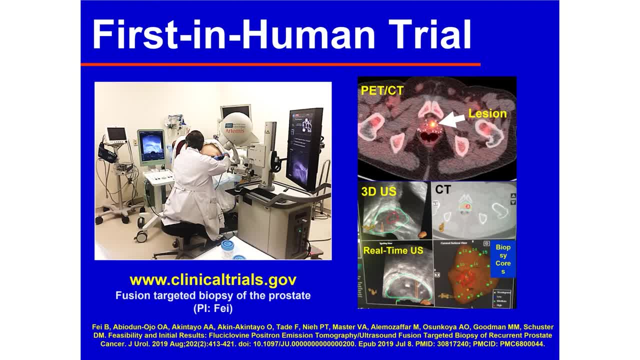 biopsy in order to improve detection biopsy in order to improve detection accuracy. so we combined a positive accuracy. so we combined a positive accuracy, so we combined a positive emission tomography pad with the emission tomography pad, with the emission tomography pad, with the three-dimensional ultrasound imaging for. 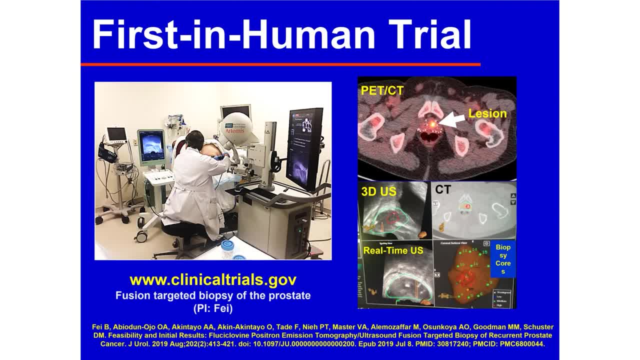 three-dimensional ultrasound imaging for three-dimensional ultrasound imaging for targeted biopsy of the prostate. this targeted biopsy of the prostate. this targeted biopsy of the prostate. this project include imaging technology project include imaging technology project include imaging technology development. mechanical design development. mechanical design development. mechanical design, software design algorithms. this is the 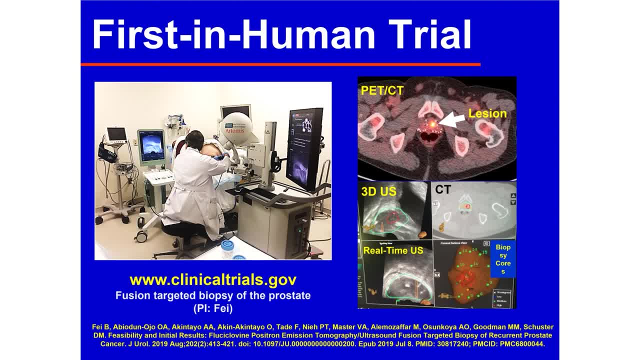 software design algorithms. this is the software design algorithms. this is the clinical setup for our patient study. clinical setup for our patient study. clinical setup for our patient study: the first in human trial of pet. the first in human trial of pet. the first in human trial of pet. molecular imaging, directed 3d ultrasound. 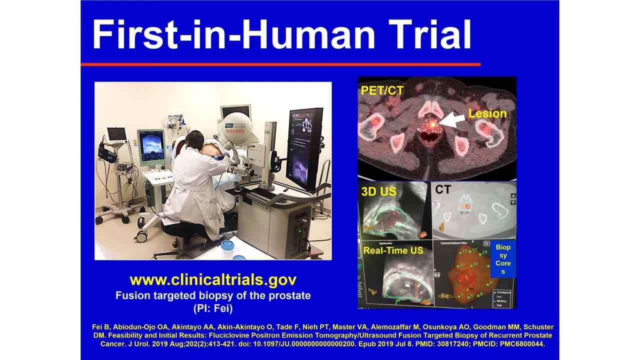 molecular imaging: directed 3d ultrasound molecular imaging directed 3d ultrasound guided targeted biopsy of the prostate: guided targeted biopsy of the prostate. guided targeted biopsy of the prostate. through this trial, we publish that we, through this trial, we publish that we, through this trial, we publish that we are able to improve prostate cancer. 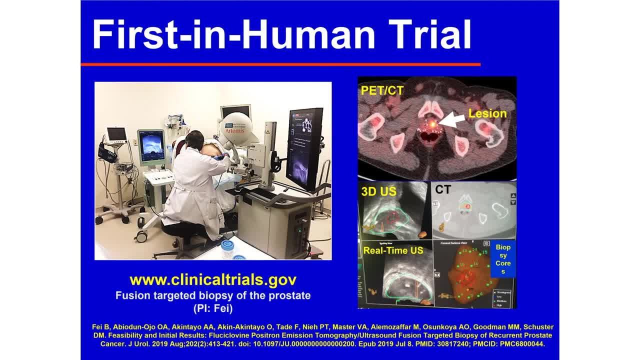 are able to improve prostate cancer are able to improve prostate cancer detection in human patient. our research, detection in human patient, our research, detection in human patient, our research have direct impact on patient care. so have direct impact on patient care. so have direct impact on patient care. so, myself, as a biomedical engineer, we are 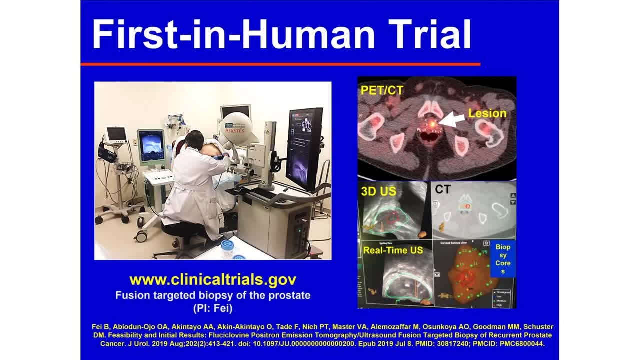 myself as a biomedical engineer. we are myself as a biomedical engineer. we are proud of being a biomedical engineer. in proud of being a biomedical engineer. in proud of being a biomedical engineer in the past decade and was a proud our work the past decade and was a proud our work. 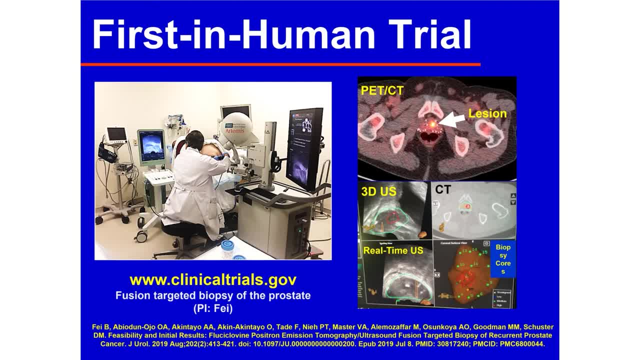 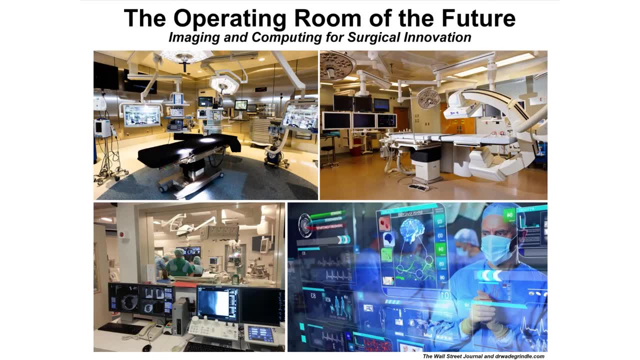 the past decade and was a proud. our work can help save life and improve human can help save life and improve human can help save life and improve human health. so I envision that imaging and health. so I envision that imaging and health. so I envision that imaging and robotics will play a critical role in 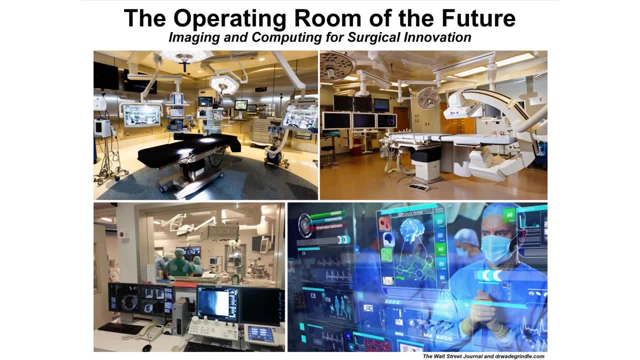 robotics will play a critical role in. robotics will play a critical role in future medicine. this is a big picture, future medicine. this is a big picture, future medicine. this is a big picture for the operating room in the future. I, for the operating room in the future, I. 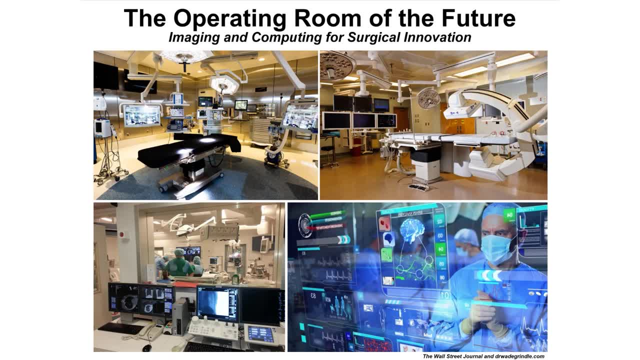 for the operating room in the future. I hope to bring advanced technology to the hope, to bring advanced technology to the hope. to bring advanced technology to the surgical room with high precision. where surgical room with high precision, where surgical room with high precision, where all the data are integrated together for 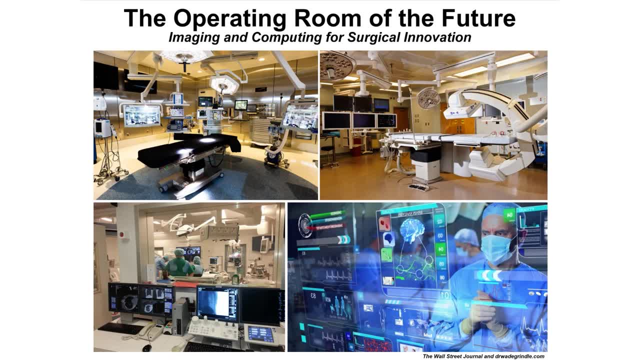 all the data are integrated together, for all the data are integrated together for better decision making. we have the better decision making. we have the better decision making. we have the artificial intelligence tools. we have artificial intelligence tools. we have artificial intelligence tools. we have augmented reality technology to see. 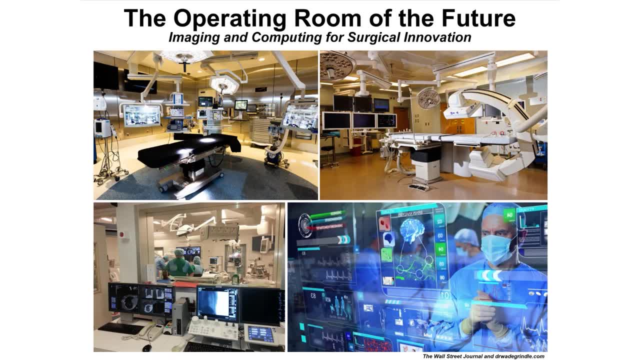 augmented reality technology to see. augmented reality technology to see through the body for precise location of through the body, for precise location of through the body, for precise location of the nation for minimally invasive the nation for minimally invasive, the nation for minimally invasive surgery. so the surgeon have the 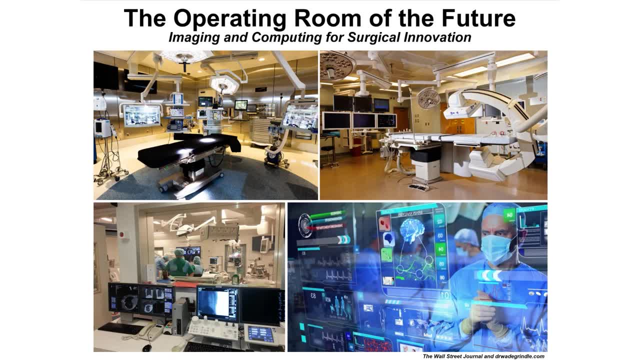 surgery. so the surgeon have the surgery, so the surgeon have the capability of detecting tumor in real capability of detecting tumor, in real capability of detecting tumor in real time at the cellular and molecular time, at the cellular and molecular time, at the cellular and molecular level. so the operating room of the 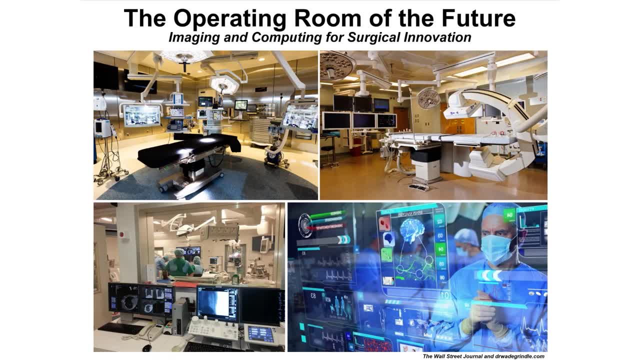 level, so the operating room of the level, so the operating room of the future. we have the integrated data future. we have the integrated data future. we have the integrated data advanced imaging technology and the advanced imaging technology and the advanced imaging technology and the computation power and to improve patient. 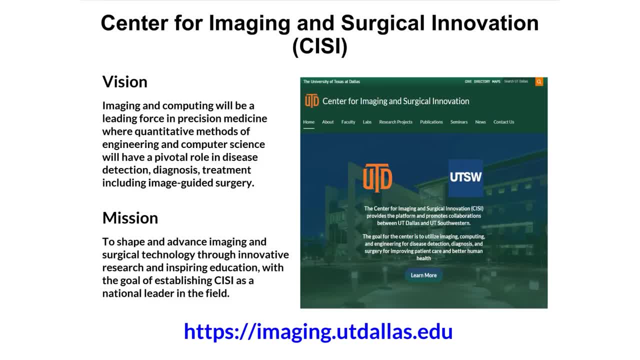 computation power and to improve patient computation power and to improve patient outcome. so, with the support from the outcome, so, with the support from the outcome, so with the support from the University and our faculty, I was able to University and our faculty, I was able to University and our faculty, I was able to establish the Center for imaging and a. 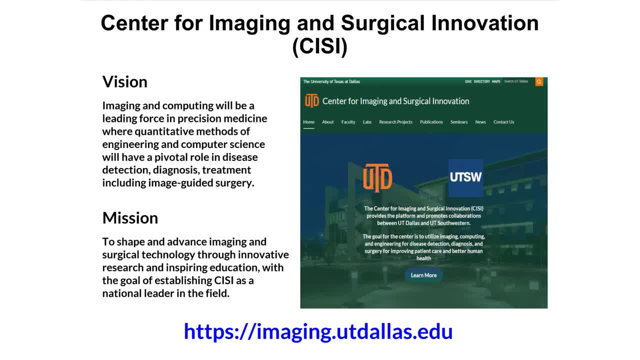 establish the Center for imaging and a. establish the Center for imaging and a surgical innovation at UT Dallas and UT. surgical innovation at UT Dallas and UT. surgical innovation at UT Dallas and UT. Southwestern, so the center is to provide. Southwestern, so the center is to provide. 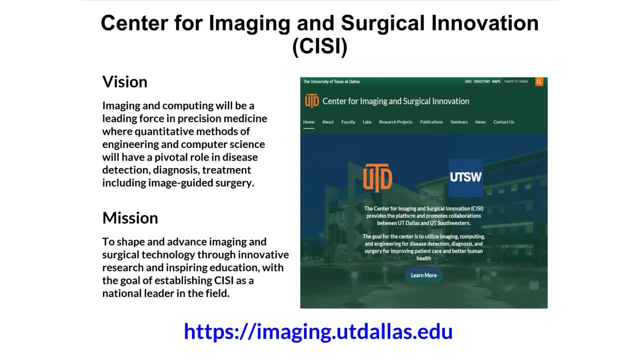 Southwestern. so the center is to provide a platform to promote collaboration, a platform to promote collaboration, a platform to promote collaboration between UTD and UT Southwestern. so I between UTD and UT Southwestern, so I between UTD and UT Southwestern. so I envision that imaging and computing will. 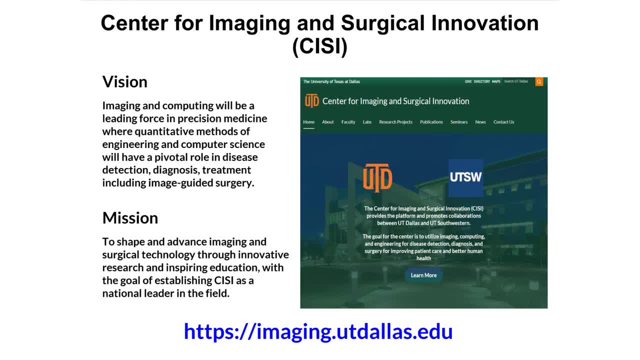 envision that imaging and computing will envision that imaging and computing will be a leading force in future precision: be a leading force in future precision. be a leading force in future precision medicine: where a quantitative method of medicine, where a quantitative method of medicine, where a quantitative method of engineering and computer science will 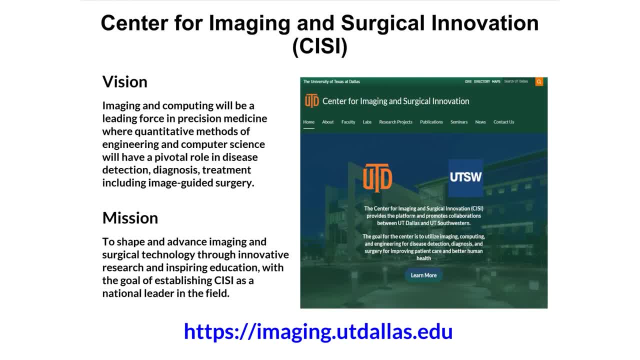 engineering and computer science will engineering and computer science will have a pivotal role in disease detection. have a pivotal role in disease detection. have a pivotal role in disease detection. diagnosis treatment, including image diagnosis treatment. including image diagnosis treatment, including image guided surgery, with this Center. guided surgery with this Center.